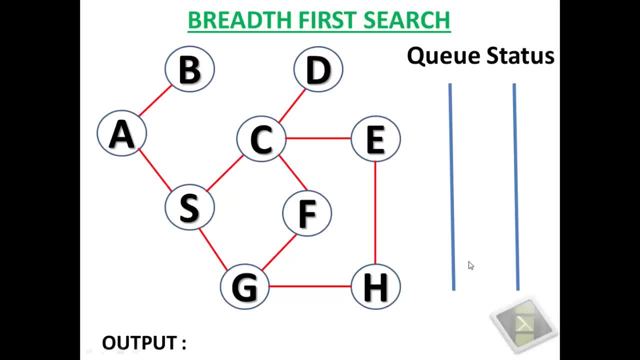 empty Q mentioned on the right hand side of the screen. We will use this Q to keep track of all the unvisited nodes of currently working node. Now, in this breadth first search, we have a concept called currently working node. Let us start our discussion with node A We. 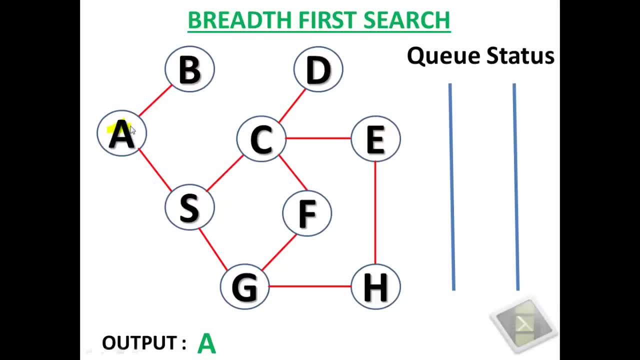 will add it to the output sequence first and we will mark it as visited. and this will be our first currently working node, which is denoted by this red arrow. Now, as per breadth, first search, We have to check all the adjacent unvisited nodes of the currently working node. Now we 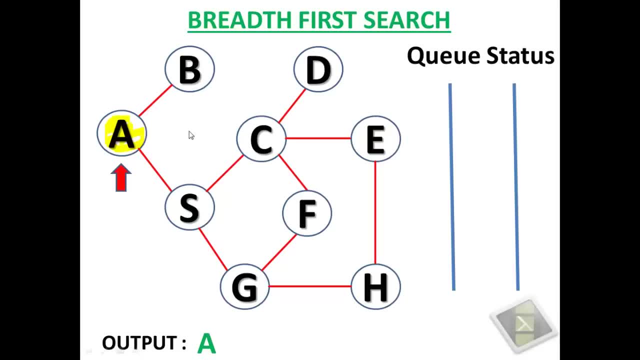 have B and S here, So we will enqueue B and S alphabetically. So we will enqueue B first and we will add it to the sequence. Similarly, and we will mark it as visited. Similarly with the S, we will enqueue it and we will mark it as visited, adding it to the sequence. 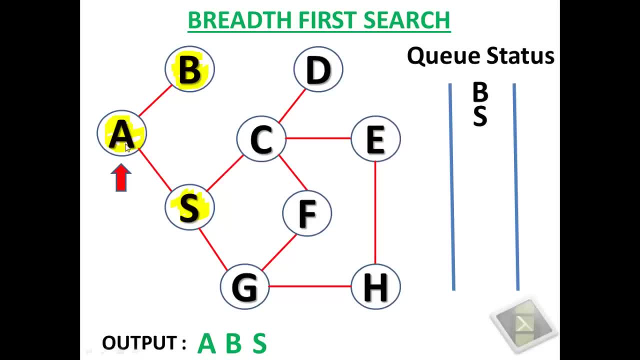 And that is it For node A. we have only B and S as adjacent nodes. Now we have to update the currently working node, So we have to check first of all the first element of the Q. We have B here. so we will update the currently working node pointing to B And dequeue B. 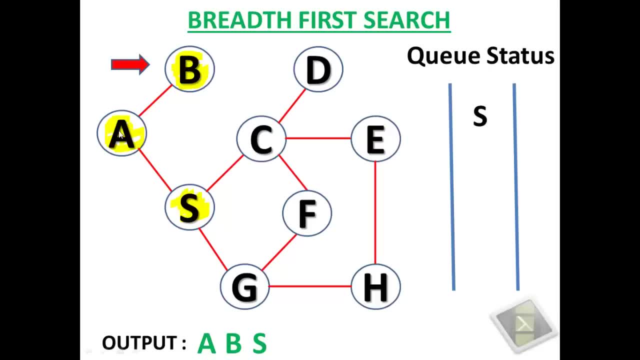 Now we see that B has only A as the current node- adjacent node which is visited already. So we have to update again the currently working node based on the top symbol of the queue. So we will update pointer to point to s and we will dequeue s. 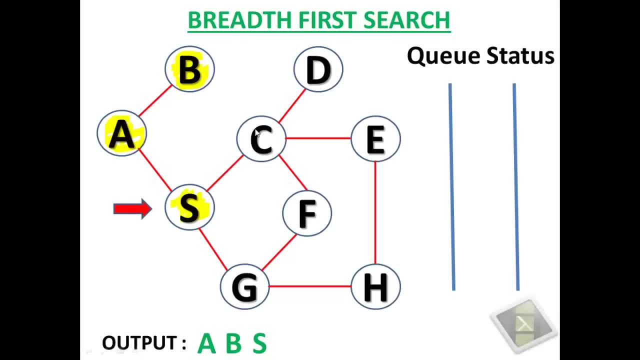 Now s has c and g as adjacent unvisited nodes. So, alphabetically, we will enqueue c first and add it to the sequence mark it as visited. We will enqueue g and adding it to the sequence marking it as visited. s has a, c and g, which are all visited, so we will update the pointer based on the top. 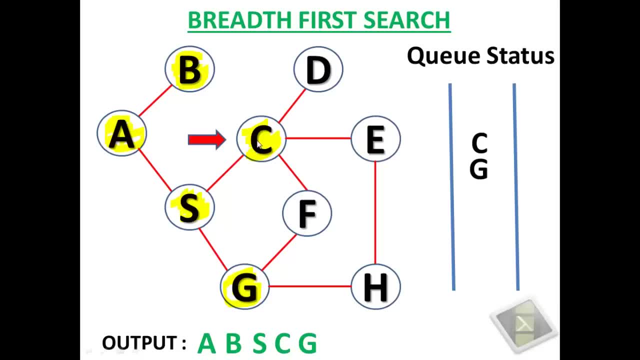 symbol of the queue. So we will update the pointer to c as the currently working node and we will dequeue c. c has d, e and f as currently adjacent and unvisited nodes, so we will enqueue d, e and f as currently adjacent and unvisited nodes.